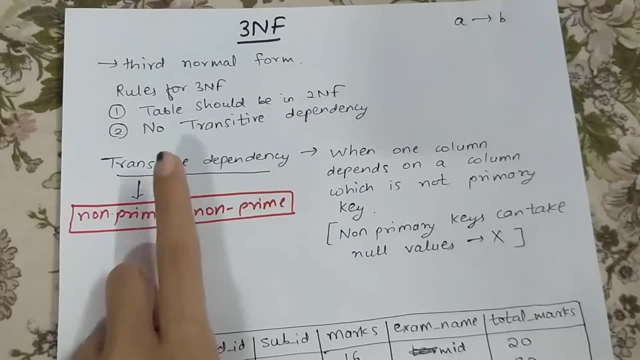 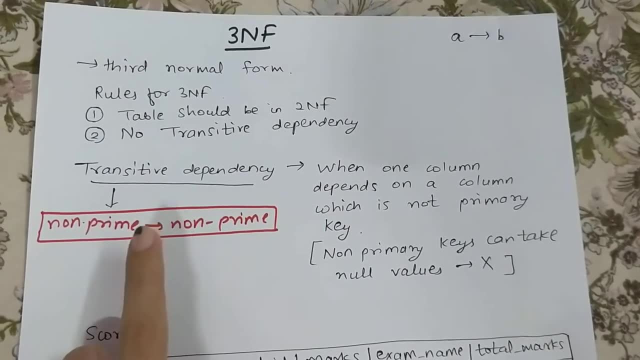 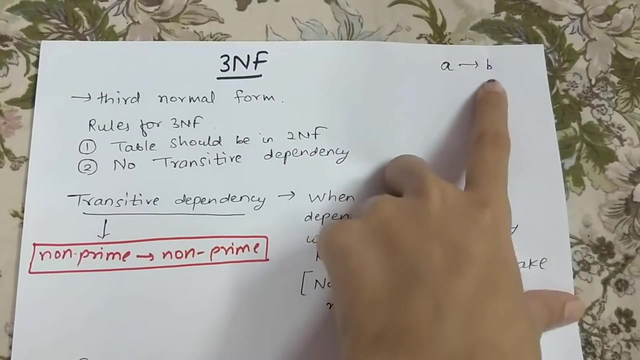 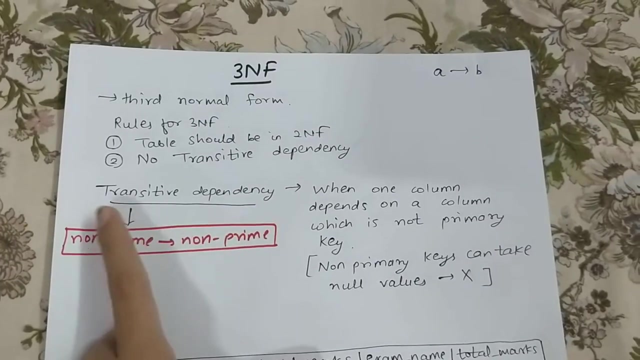 So now to understand what transitive dependency is, let's understand it. So, basically, transitive dependency is when a non-prime depends on another non-prime. When I write a arrow b, it basically means that b depends on a. So when I am saying non-prime, arrow, non-prime, it means when a non-prime attribute depends on another non-prime attribute. 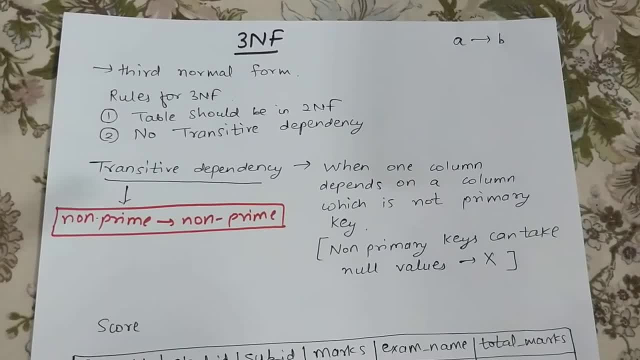 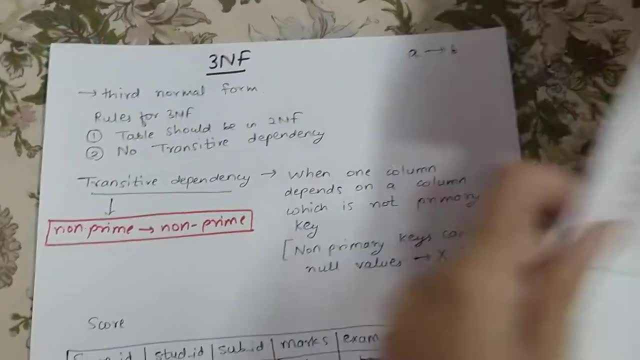 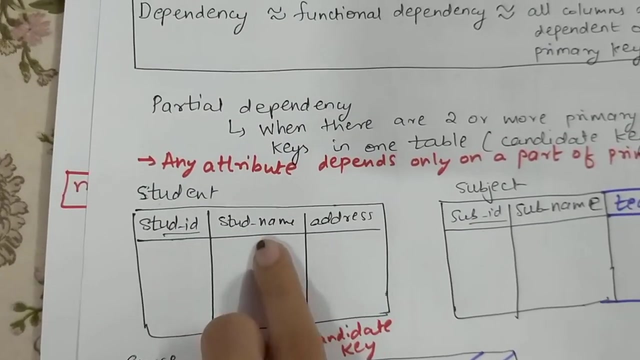 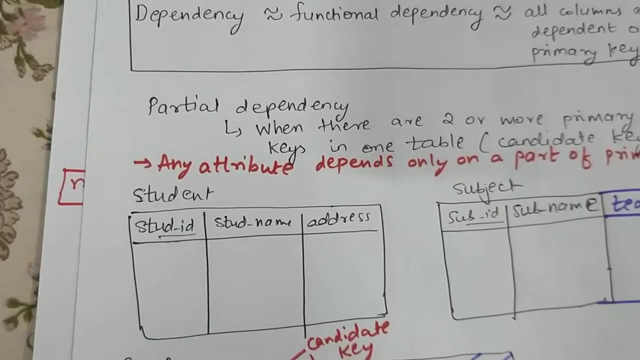 Now, what is non-prime attribute? Now, what are prime attributes? Prime attributes are prime. They are the primary keys on which all the other columns depend. Now, for example, this was a table, student table. Now, student id is a prime attribute, prime key because it is a primary key. The other column, that is student name address. these are non-prime attributes because they are not prime. Basically they are non-prime because they are not prime keys. 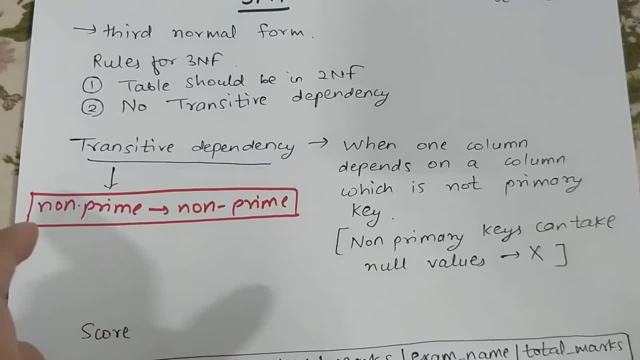 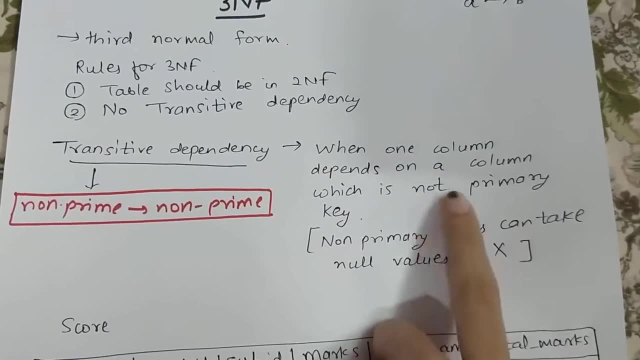 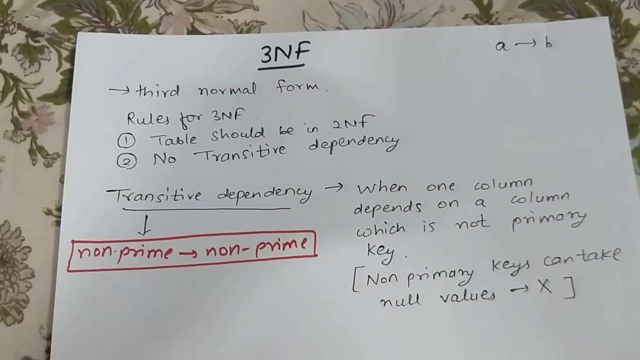 So when a non-prime depends on another non-prime, that is when transitive dependency comes into existence. So when One column depends on a column which is not primary key, okay, That is transitive dependency. So non-prime keys can take null values, okay. 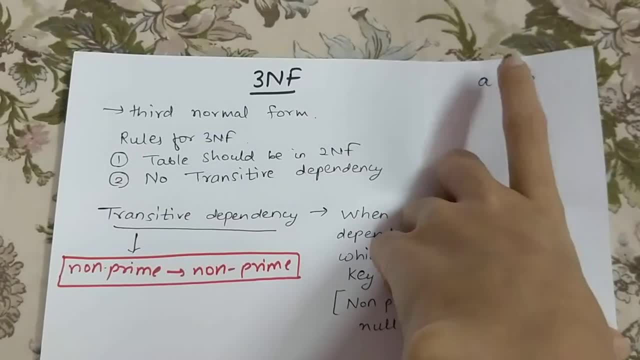 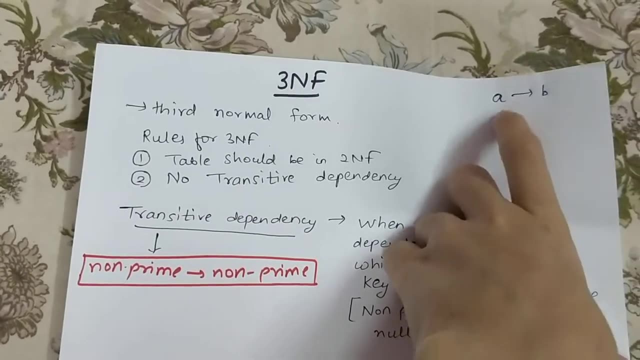 So, basically, when this is a non-prime and it is dependent on another non-prime and this non-prime values, as it is not a prime value, prime key, so it can take null values. So basically this can have null values. So, for example, this is 0.. 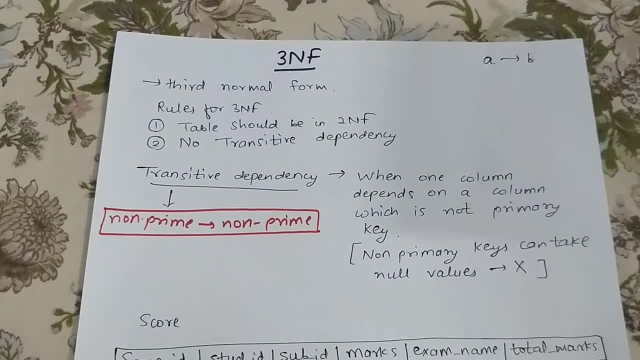 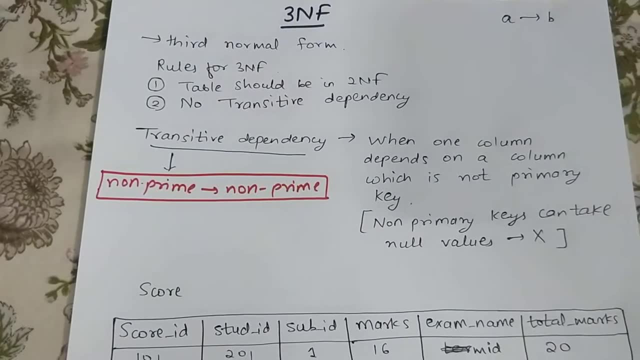 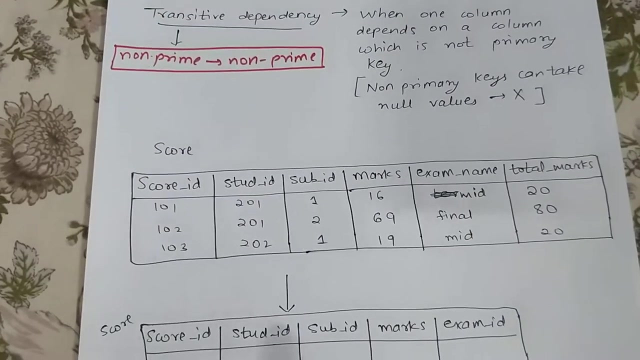 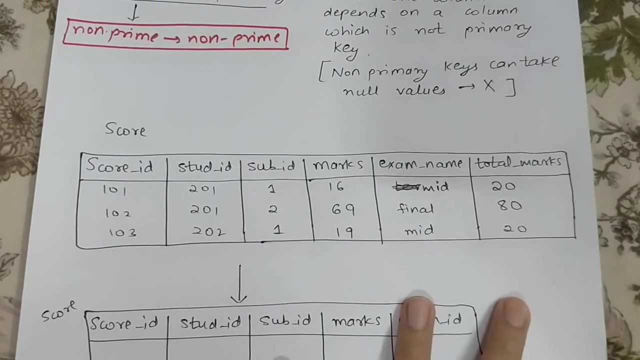 So in this case, this will depend on a null value, 0 value, which is not allowed, and that is why transitive dependency should be removed, Because all the columns should only depend on primary keys and not on non-prime keys. Alright, so let us understand it with an example. Now, this is a score table, so it has score id, student id, subject id marks, exam name, total marks. 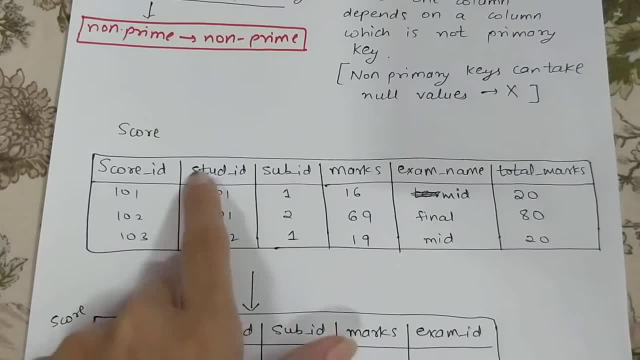 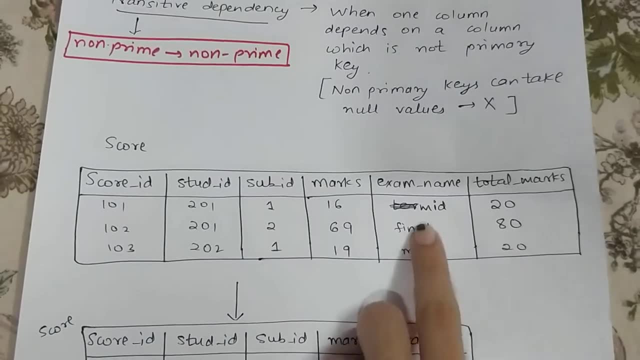 So score id. So these are the student student id and student number. student ids, subject ids, marks, whatever the marks the particular student gets. and these are the exam names. now. exam name could be mid-exam or final exam. okay, now if it's a mid-exam, total marks: 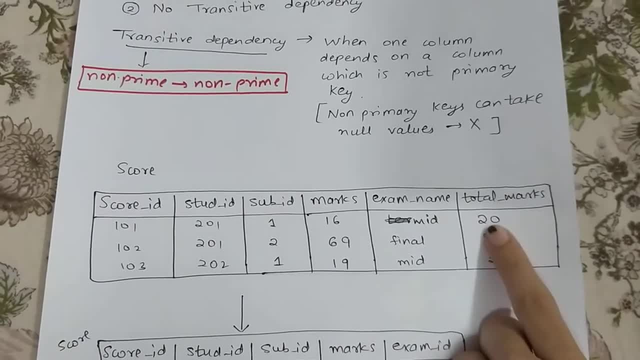 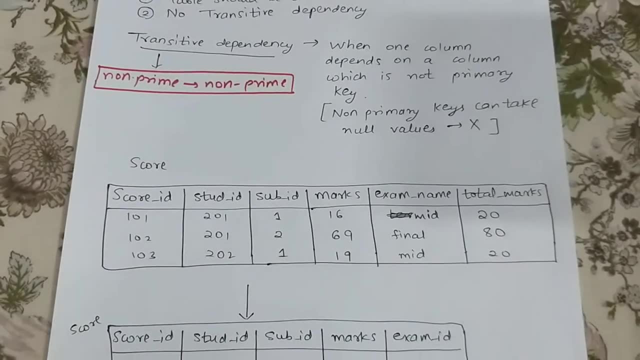 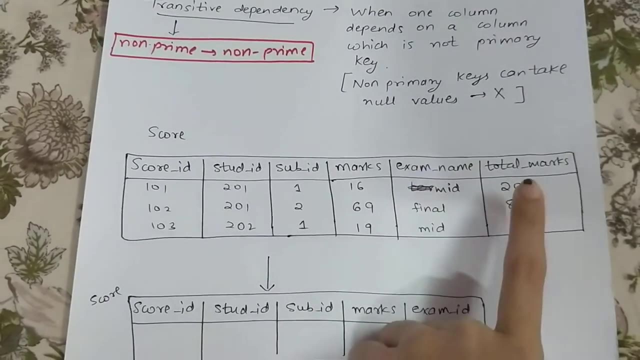 to uh, total marks would be out of 20. okay, and if it's a final exam, it will be. the total marks would be 80 and if it's a mid-exam, total marks would be 20. so, as you can see, the total marks are dependent on this column, so this column is basically dependent on this column. 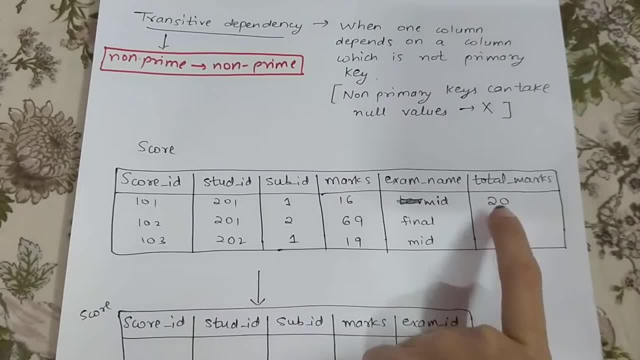 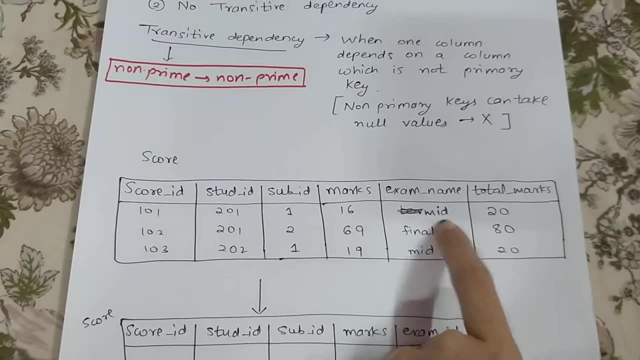 because whatever the values are going to be here, okay, if it's going to be 20 or 80, it will depend on the values which will be over here in this column. if it's a mid, here there will be 20. if it's a final final exam, here there will be 80. so, basically, this is a non-prime key and 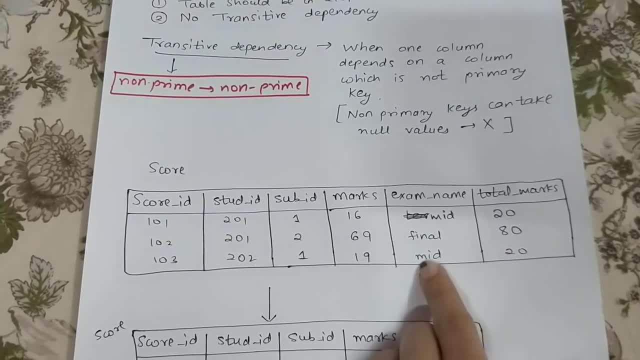 this is a non-prime key and this non-prime key is dependent on another non-prime key, non-prime, dependent on another non-prime, so basically transitive dependent on another non-prime key. so basically transitive dependent on another non-prime key. 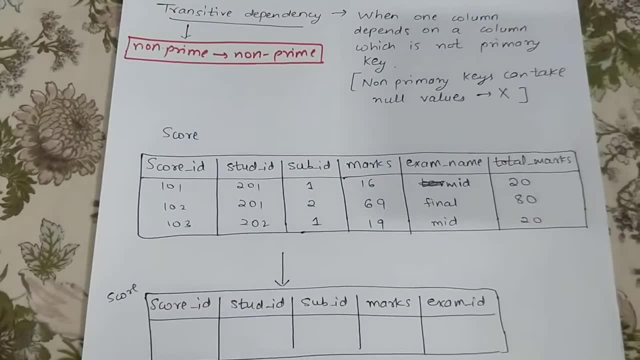 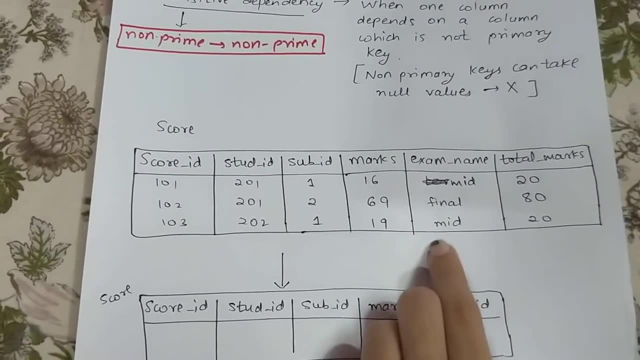 dependent on another non-prime key. so basically, transitive dependent on another non-prime key is here, okay. now, as this is a non-prime value, okay, so it can have values which are null and hence, if here there will be a null value, this will also become null and this, this will. 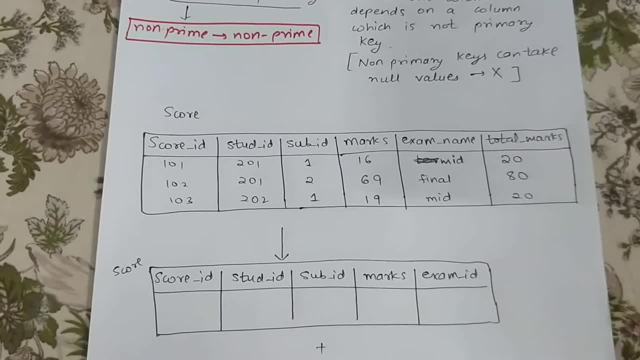 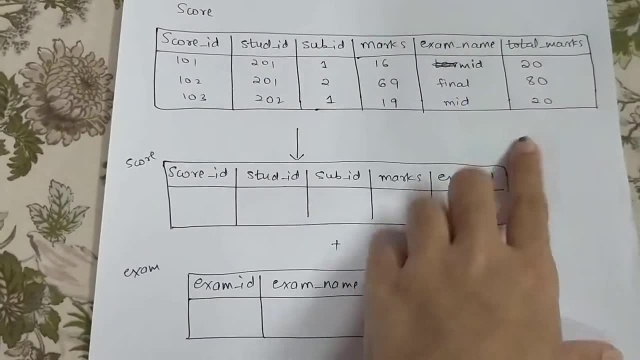 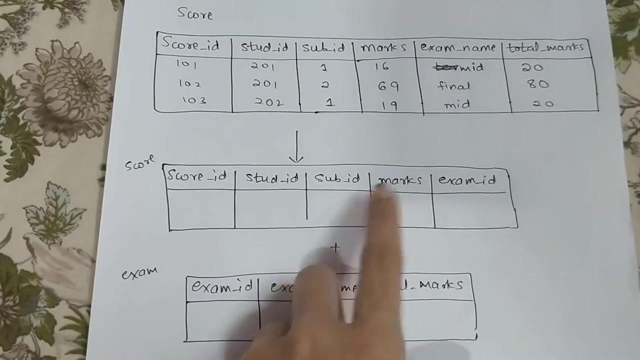 create. this will create an issue and hence three nf should be there. okay, so this is how we can change. this is how we can remove transitive dependency. we will just convert into two tables transitive dependency. we will just convert into two tables. so this one score table where there is score id, student id, subject id, marks id and there will be an exam. 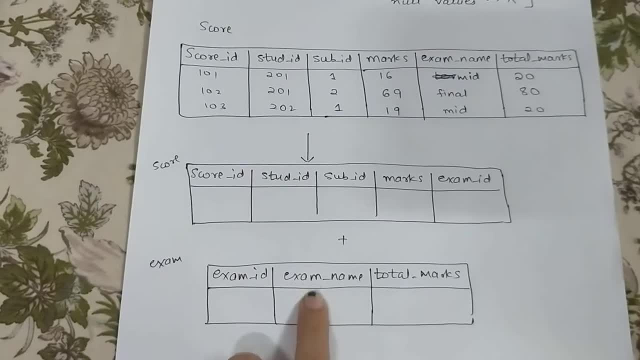 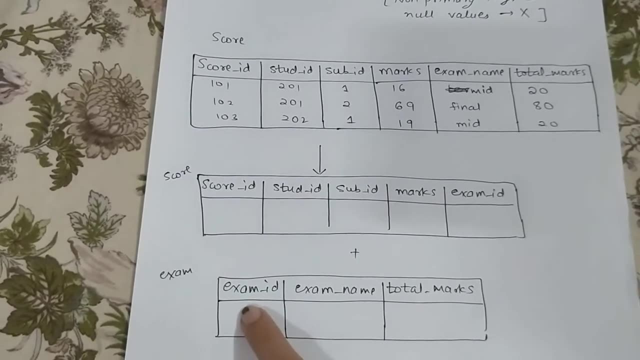 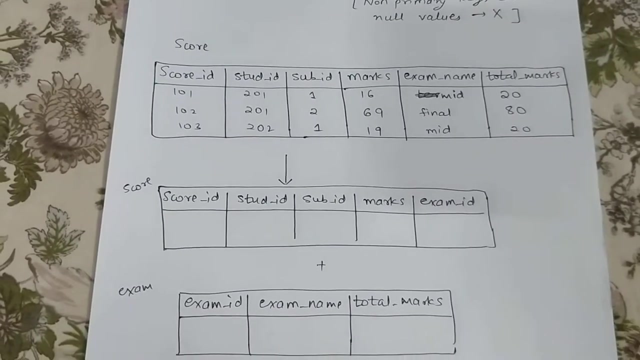 id, which will link it to another table: exam id, which is exam name, total marks. so here total marks will only depend on exam id. so whatever the exam id will be there, so these two will depend on it and hence there will be no transitive dependency. and this is how we will remove it and bring it in. 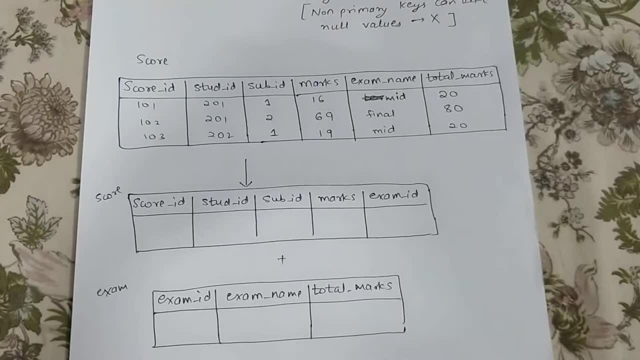 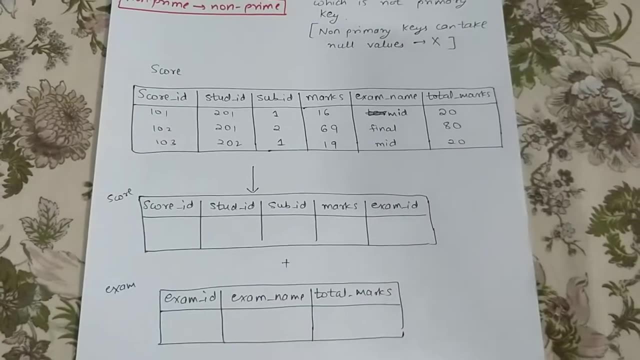 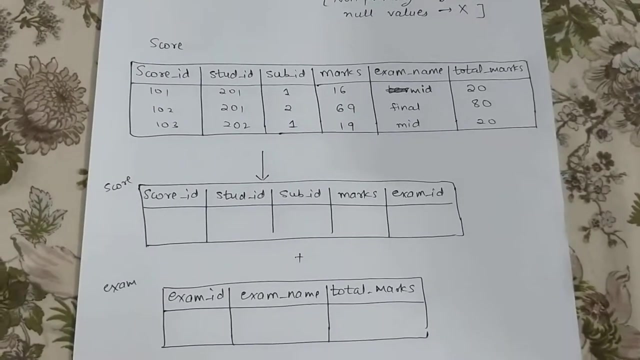 the 3nf form. okay, basically, in normalization we just make a bigger table into smaller tables and add primary keys and link them together. this is what normalization is. uh, and all the other, all the forms- 1nf, 2nf, 3nf, all of them. they just have different rules and that's it. but the basic thing. 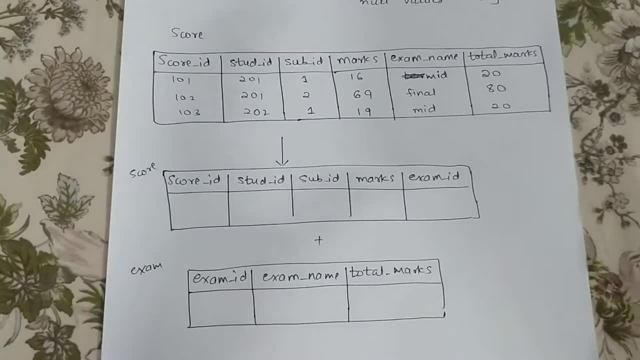 is dividing into dividing the bigger table into smaller tables. okay, thank you for watching.